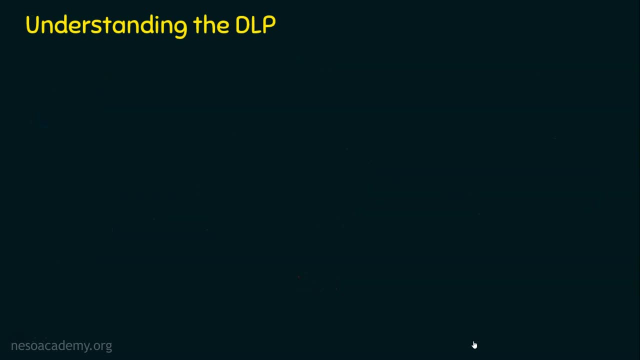 understanding the discrete logarithm problem. We know very well this modular arithmetic is also called as clock arithmetic. Let's take a prime number: 17.. Just imagine there is a clock with 17 units. So we can see that the clock is from 1 to 17, where 17 is a prime number and we 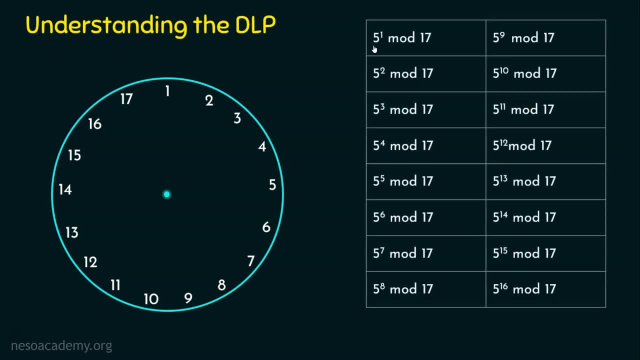 are taking a number called 5.. Can you see here the number: 5- power 1, mod 17,. 5- power 2, mod 17. up to 5- power 16, mod 17 is performed. Can you just recollect what concept is this? Just recollect? 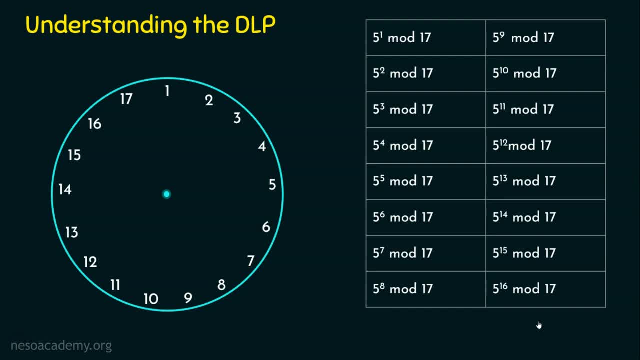 the concept of primitive roots. What did we do there? We took a prime number and we took the primitive root of this prime number. If 5 is a primitive root of the prime number 17,, then 5 power 1 mod 17,. 5 power 2 mod 17 up to 5 power 16 mod 17.. 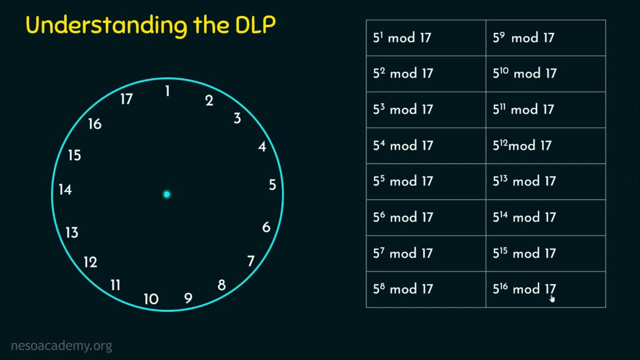 That is, if 17 is the prime number which is denoted as p, then 5 power p minus 1 mod p, that is 5 power 16 mod 17, will give unique result. Let's start with 5 power 1 mod 17.. 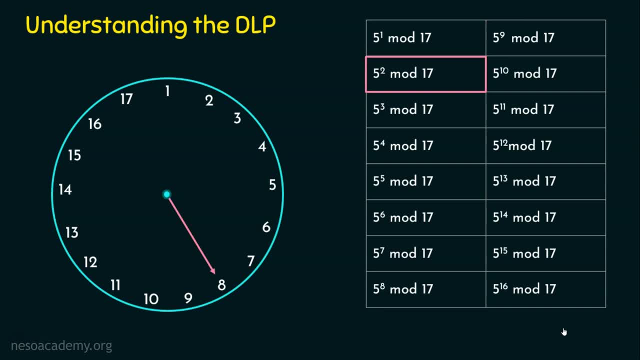 5 power 1 mod 17 is 5.. 5 power 2- mod 17 is 8.. 5 power 3- mod 17 is 6.. 5 power 4 is 13.. 5 power 5- mod 17 is 14.. 5 power 6 gives 2.. 5 power 7 gives 10.. 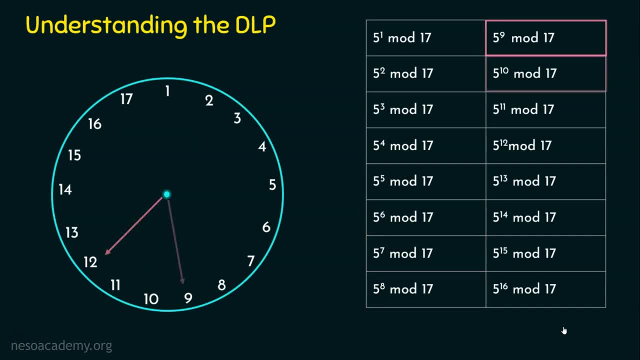 5 power: 8 gives 8.. 5 power: 7 gives 8.. 5 power: 8 gives 8.. 5 power: 9 gives 12.. 5 power: 10 gives 9.. 5 power: 11 gives 11.. 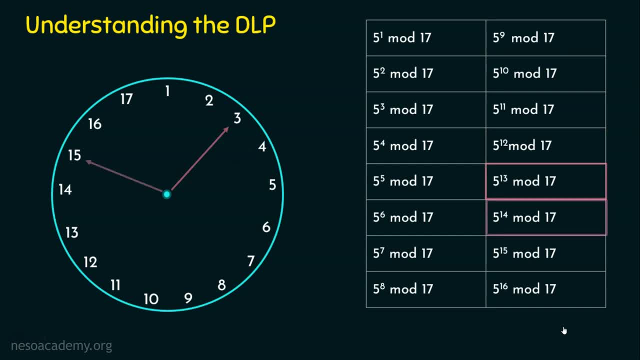 5 power 12 gives 4.. 5 power 13 gives 3.. 5 power 14, mod 17 gives 15.. 5 power 15, mod 17 gives 7.. And 5 power 16, mod 17 gives 1.. 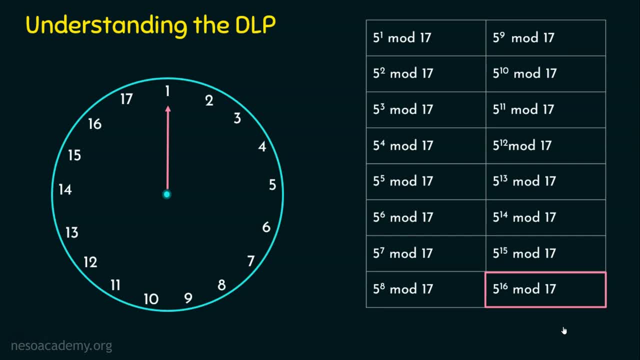 If you observe, in this entire scenario the results are uniformly distributed. So from 5 power 1 to 5 power 16 mod 17,. we got unique result And that is why we said 5 is a primitive root of the prime number 17.. If things are not clear, let's see this in a different way. 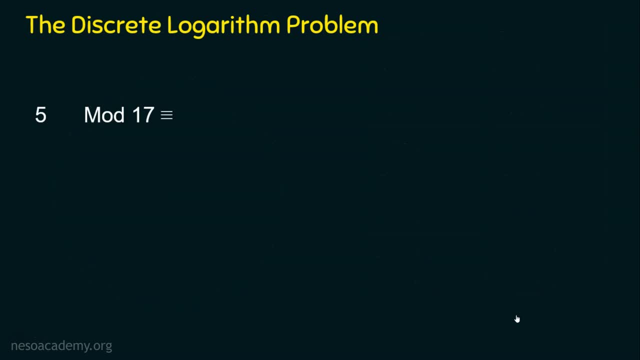 Say we are going to compute 5 power x mod 17.. We know 17 is a prime number and 5 is a primitive root. When we will say 5 is a primitive root of the prime number 17,. if 5 power 1 mod 17 to 5 power 16 mod 17 gives unique results. Say 5 power 1 mod 17 gives 5.. 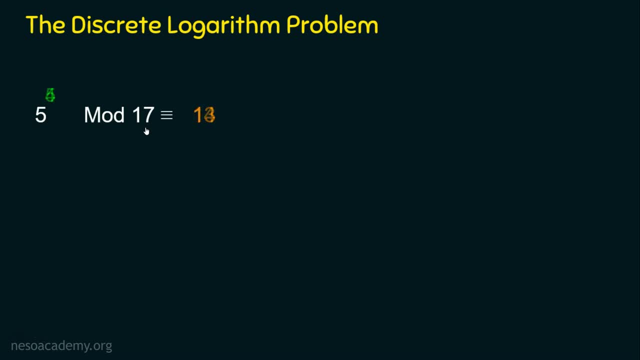 5 power 2 gives 8.. So when we carry out this operation we get unique results. So from 5 power 1 to 5 power 16, we are getting the results that is actually uniformly distributed. So that is the important property of the prime number and the primitive root. 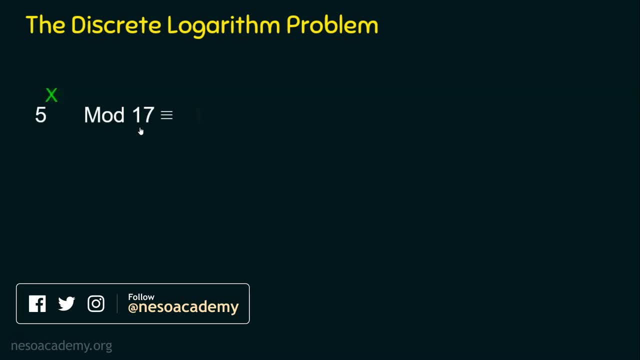 So what we understand from this is that when we deal with 5 power x mod 17 and when we start giving the numbers for x, then we can see the result that is equally distributed. Say this: x mod 17 is equal to 5 power x mod 17.. 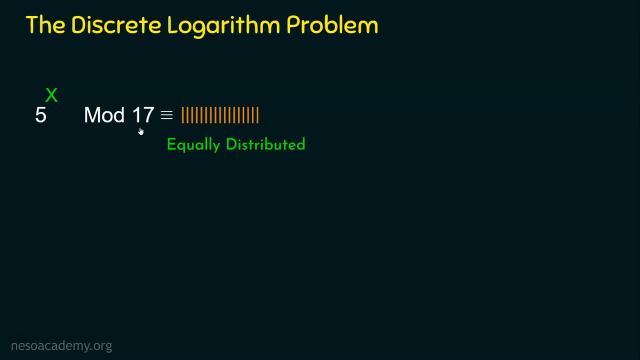 So x can be from 1 to any range, But still the prime number is 17.. So this is applicable only when there is a prime number and we have a primitive root for that prime number. So we call this number 5 as a primitive. 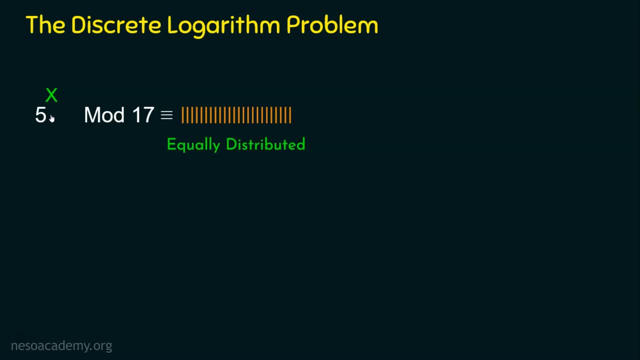 root or generator. So it's clear that if we want to compute 5 power x mod 17, it is easy to do it. Say you are given with a number x, and computing 5 power x mod 17 is easy. 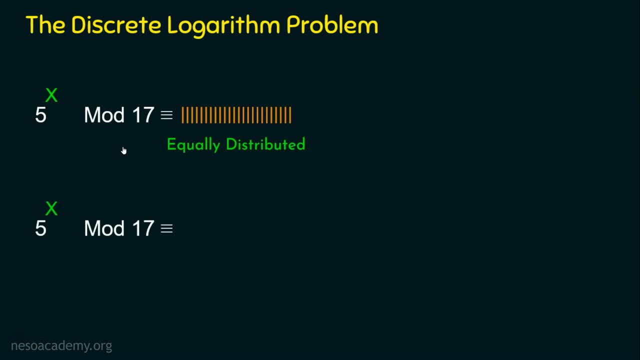 But think of the reverse situation. Say you are having 5 power, x mod 17 and you are given, with the result 12.. Now finding what is this value of x is tough, because x can be 9.. 5 power- 9 mod 17. 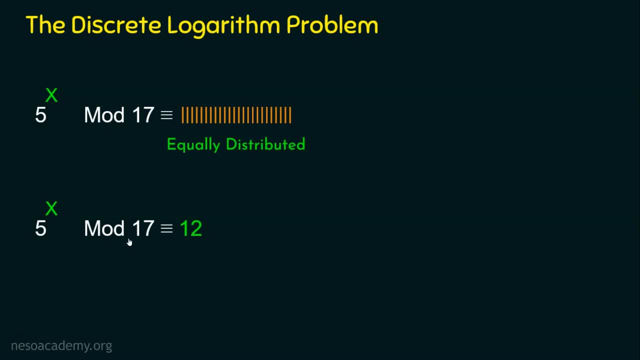 will be 12.. 5- power 25, mod 17 will be 12.. 5 power 41, mod 17 will be 12.. 5 power 57, mod 17, will be 12.. 5 power 73, mod 17 will be 12.. And there can be any value for this x. 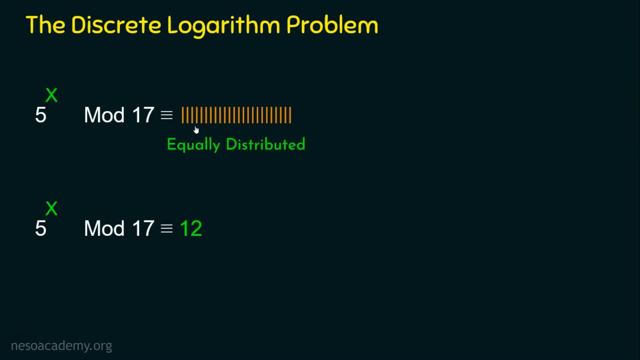 If x is given, computing 5 power, x mod 17 is easy, But if 12 is given, then finding the value of x that resulted in this value, 12, is difficult. So that is what I told you. It is easy in one. 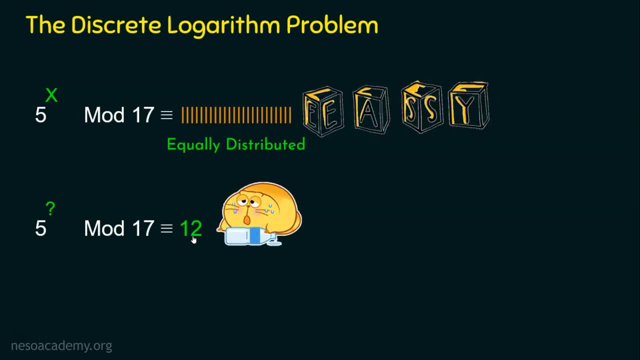 direction, but it's hard in the reverse direction. So this is what the important property of a one-way function. I think now you can understand why it is called as a one-way function. Just correlate this with the coffee analogy which we dealt in the 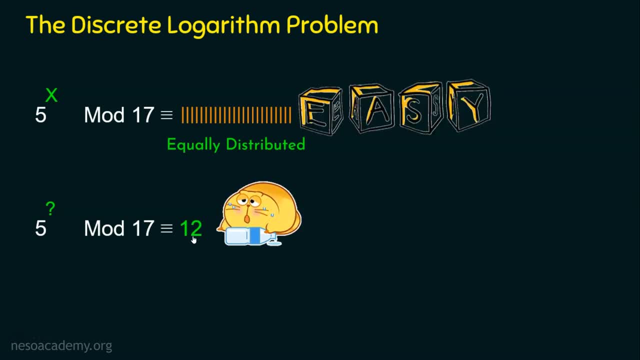 initial part of this lecture. So preparing coffee is easy, but reverting this is tough. So that's the important property of a one-way function. I think now you can understand this. So computing 5 power x mod 17,. if the value of x is given, then it is easy in one direction. 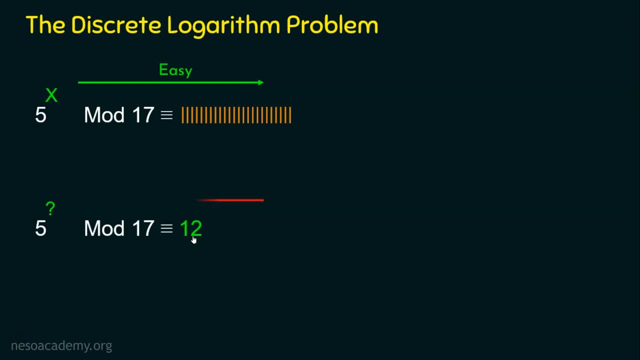 But think: if 12 is given and if you are required to find what is the value of x, it is hard in the reverse direction. This is what a one-way function is. Let's see the theoretical proof. so we are going to compute, for example, g power, x mod p, where g is the primitive root of the. 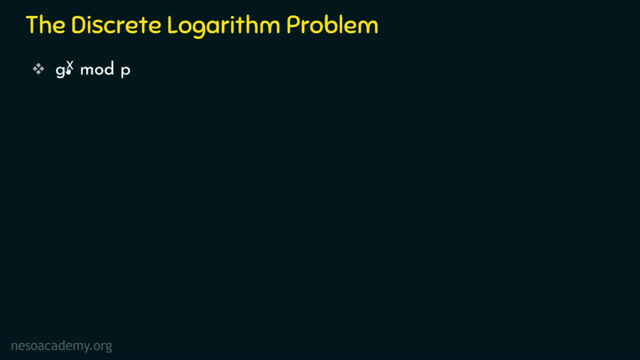 prime number. p and x can be any number, but computing g power x mod p is obviously easy in one direction. Let's take an example. Let's take 2 power x mod 7, which is equal to 4.. Now what value of x will give the result 4?? If we take x is equal to 2, then 2 power 2 is 4, 4 mod 7 is 4.. 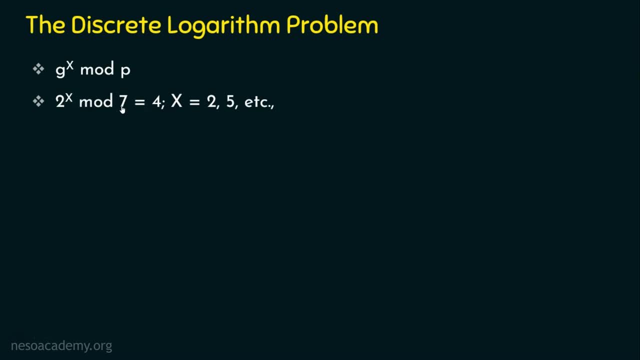 take 5, 2 power, 5 is 32.. 32 when it is divided by 7, we get 4 as the result. So there can be any number of values for x possible If 4 is given. it's really tough to decide what is the value of. 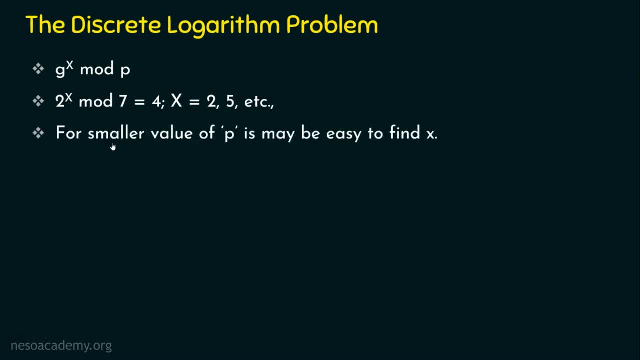 this x Can be 2 or 5 or anything. For smaller value of the prime number p, that is, for smaller values of this prime number, it may be easy to find x. But think, if the prime number is a large prime number or a very large prime number, then finding this x is hard. If the prime number p we 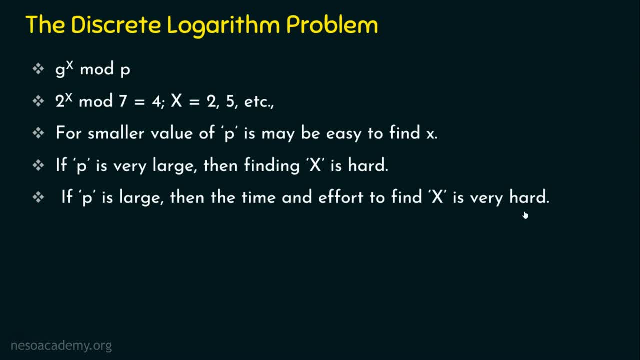 take is large, then the time and effort to find this x is very hard. So that's the logic behind one-way function. So the strength of a one-way function is depending on how much time it takes to break it. If you take a large prime number- p, even if you know what is the primitive root,